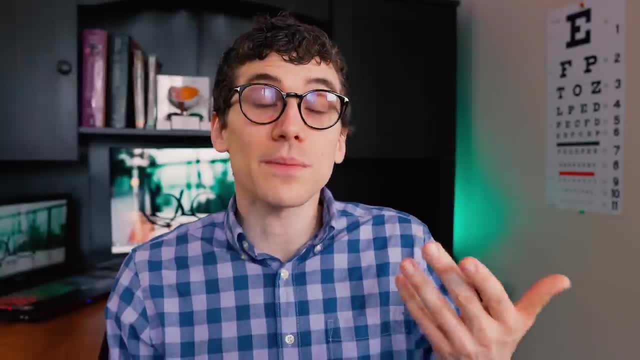 even if you don't have one, Freud Sanitarium will still be worth it once you can. père the get. Wow cool. These cameras don't want blind see-through folks. They're not going as far and I've heard there's kind of a sense of 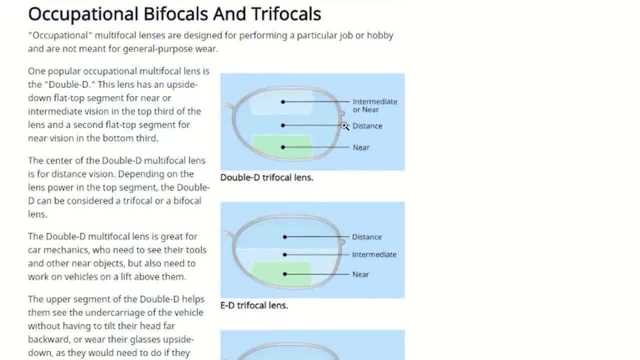 something where there's nobody looking at you, but they're trying to force you out of being able to actually spot who you're looking at and get you closer and closer. Won't they find that interesting enoughSEP somebody who maybe works underneath cars like an auto mechanic or an electrician? And as far as price for glasses. you can go from anywhere, from the cheap bargain bin low quality pair of glasses that you can find in some optical shops online to the most expensive, extravagant pairs of glasses that are out there. Some celebrities are even known to pay $10,000 or more for a single pair. 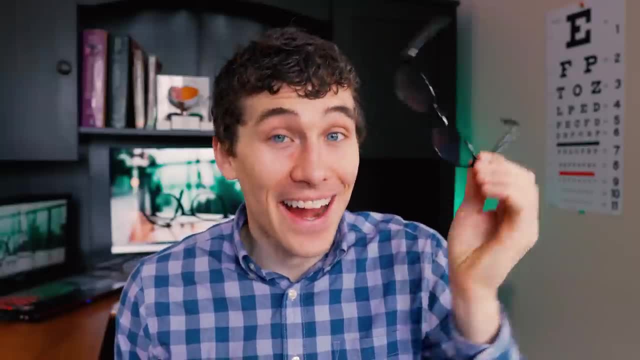 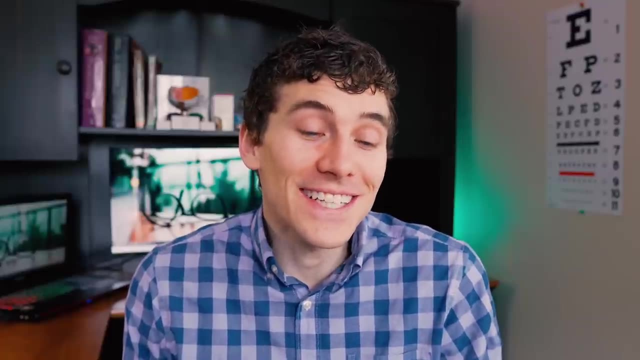 of designer glasses. Now, as far as contact lenses goes- and yes, I am wearing contact lenses underneath these glasses- I just want to give you a heads up. I am pretty biased toward contacts just because contact lenses changed my life when I first got them, when I was 13 years old and 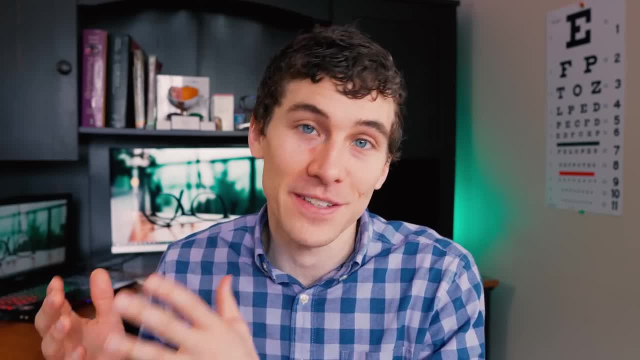 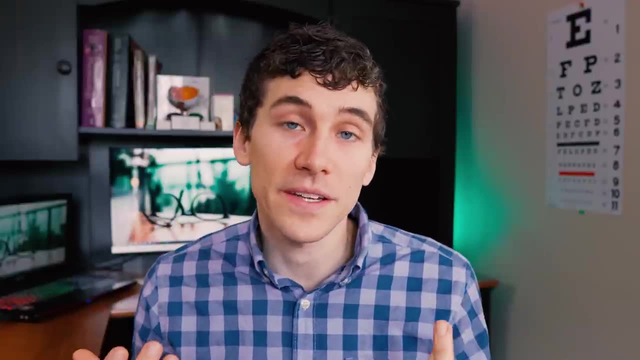 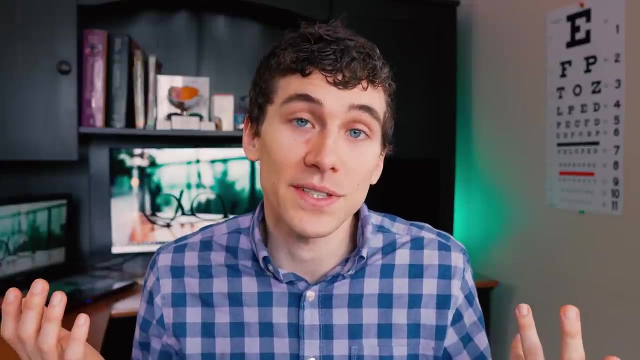 honestly definitely contributed to me even becoming an eye doctor in the first place. Some of the reasons I love contact lenses versus glasses is that contact lenses give you the freedom of not having to wear anything on your face, especially really good for social engagements as well as sporting activities. That's, in fact, the reason I got into contacts when I was 13. anyways, because I wanted to play sports, and it's kind of hard to play sports with thick Coke bottle glasses. Wearing contact lenses also allows you to wear non-prescription sunglasses a lot easier, which is something that I absolutely love to do. And then also contact lenses take. 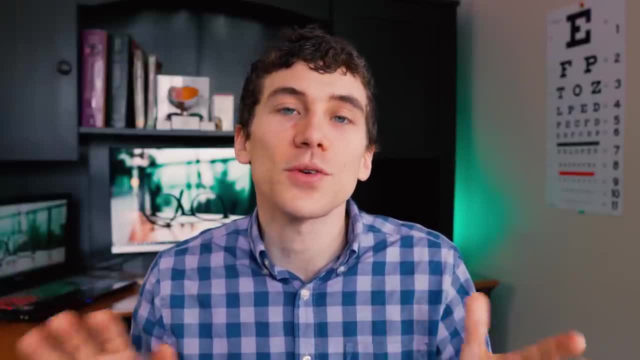 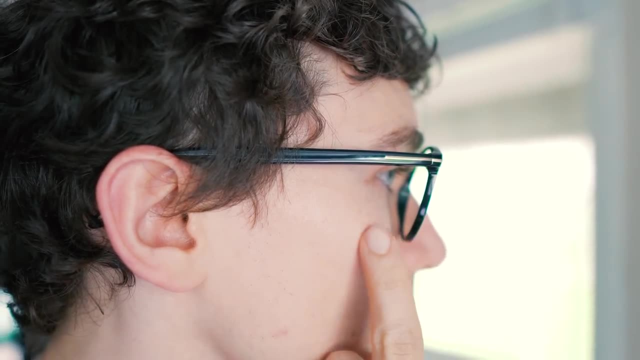 away some of the motion sickness and kind of distortions that you can get from wearing glasses lenses- Because when you're wearing glasses your glasses sit about 12 millimeters in front of your corneal plane And when you look around through a different part of the lens and shift your eyes, 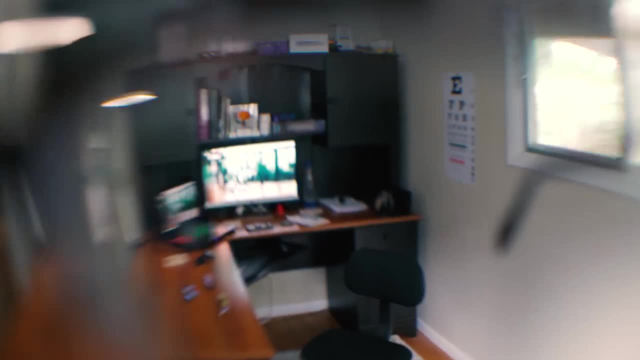 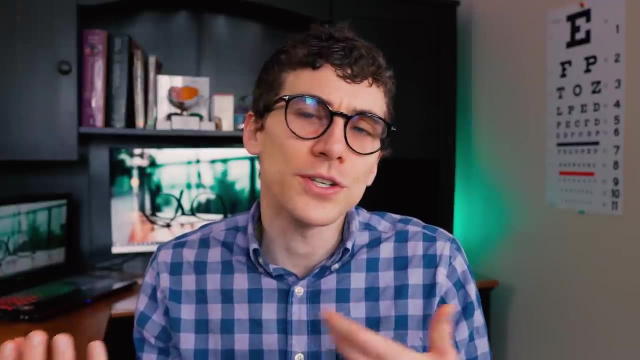 around. you're going to look through that different part of the lens and that's going to have a prismatic effect that we call Prentice's rule, And that prismatic effect can kind of give people this sense of motion or distortion in their lenses, especially for people with high amounts. 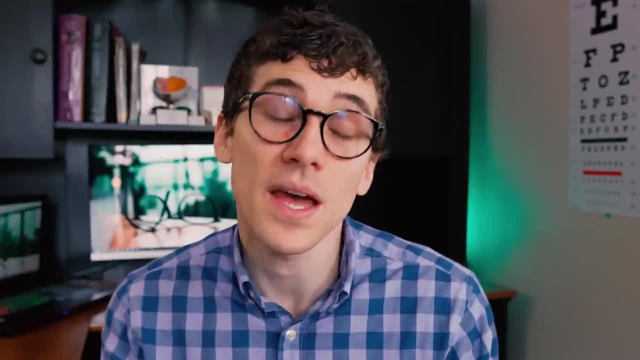 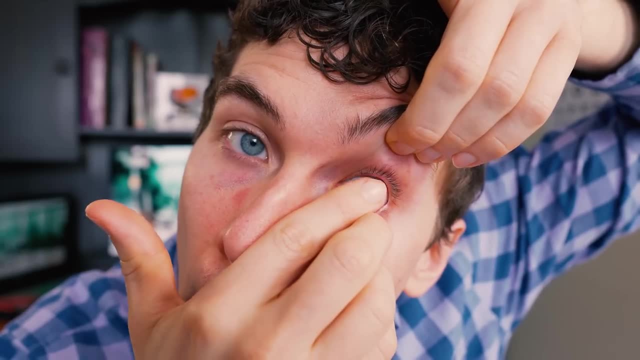 of higher powers or even higher amounts of astigmatism, They're more likely to notice that motion sickness feeling. But with contact lenses, since the lenses themselves are physically touching the eye, when you shift your eyes around, you're looking through the same part of the lens all the. 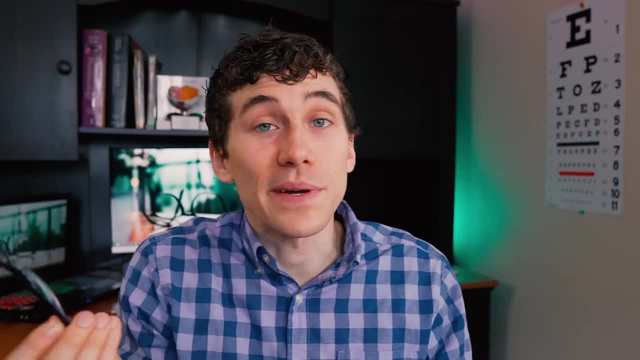 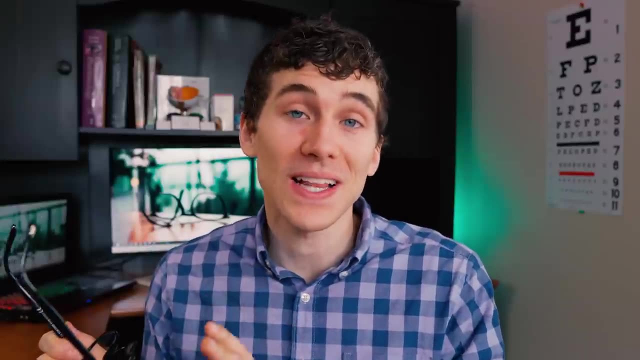 time, And so you don't get that same kind of prismatic effect. And another benefit is that with contacts you don't have to deal with looking through a frame and part blocking part of your vision all day Now a frequent question I get about glasses versus contact lenses is: 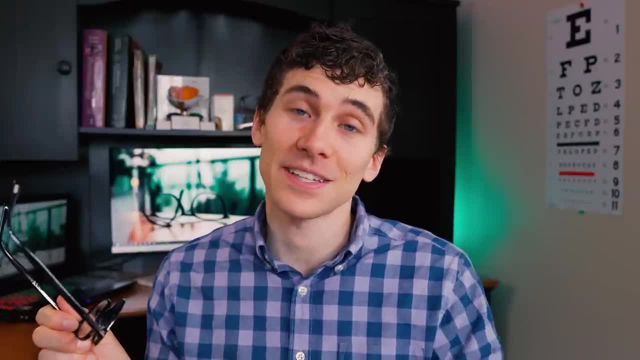 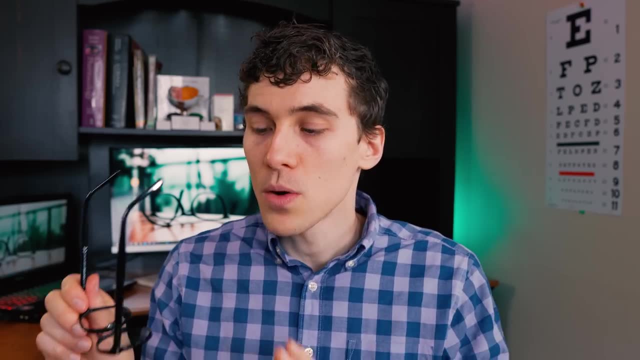 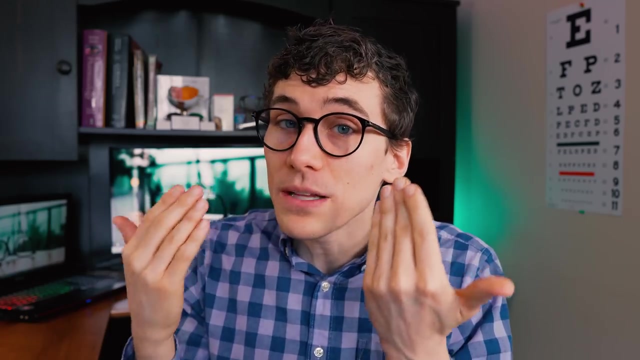 has to do with the power of the lenses in your glasses versus the contacts. Now, glasses lenses power are not necessarily going to be the same as a contact lens power. The reason for that has to do with how your glasses sit in front of your face. Again, they're usually about 12 millimeters. 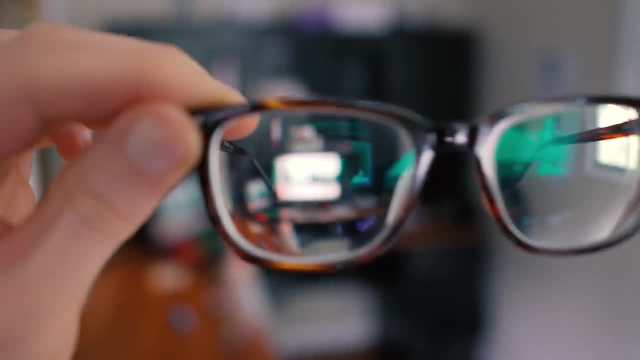 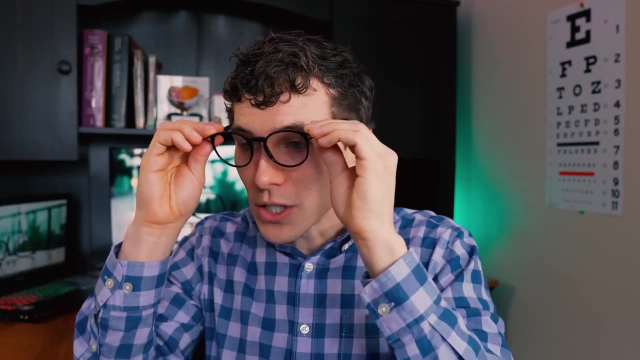 in front of the cornea. And if you've ever picked up your glasses and move them closer to your eyes and kind of move them, trombone them, back and forth, you'll notice that the power seems to change. And that's because the closer you bring the lenses to your eyes, the closer your eyes. 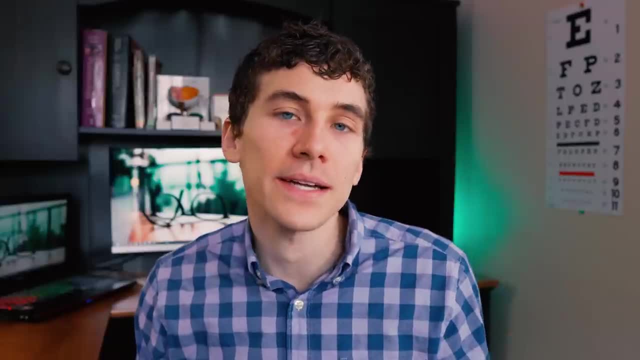 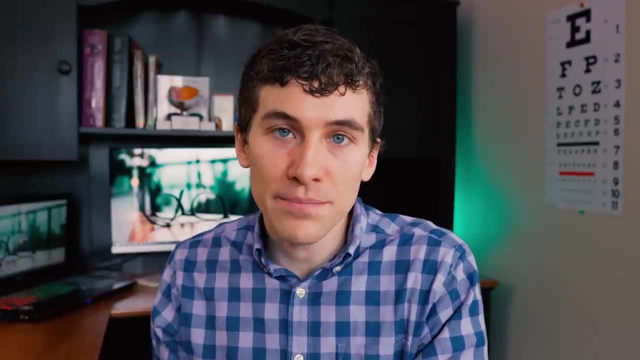 to your eye, the more kind of negative power you're adding to those lenses. So for people who have a stronger prescription in eye care, we usually reduce the amount of negative power or we add more plus power when the contact lenses are getting moved from the 12 millimeter of your. 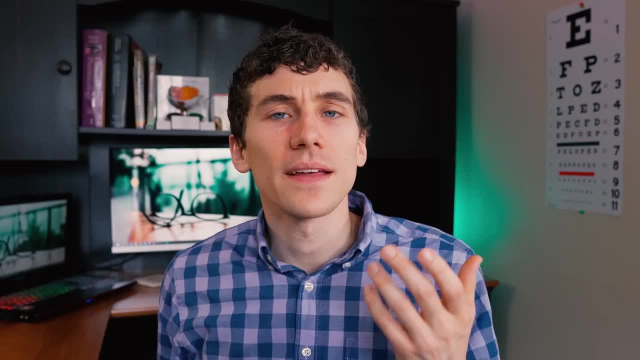 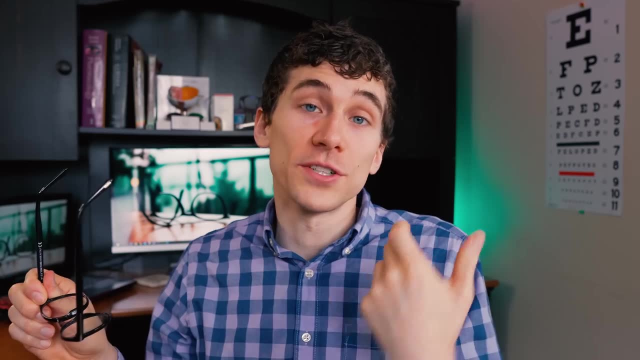 glasses to directly onto the cornea, as with contact lenses, And this adjustment that your doctor factors in is based on two things: the power of your glasses, because the higher power you have, the more of adjustment needs to be made, as well as where you're looking through your 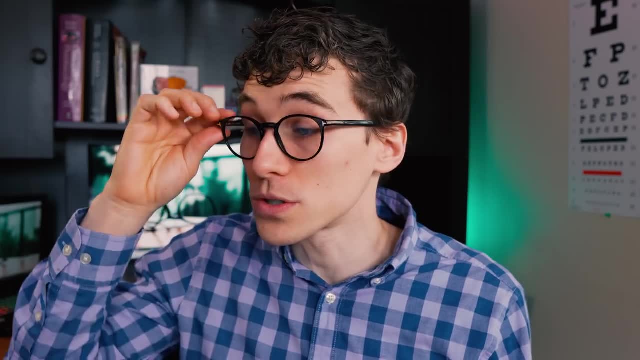 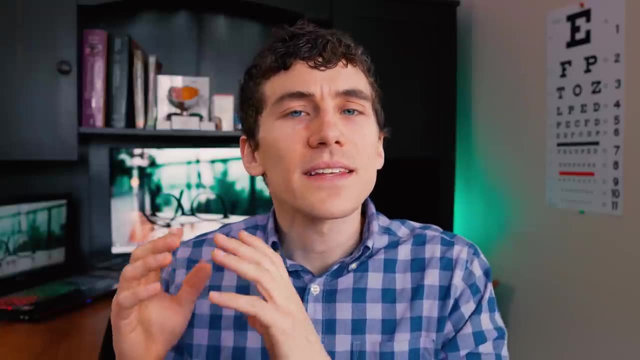 glasses are typically sitting on your face. Is it at 12 millimeters, or is it further down, at 14 or 15 millimeters? That does make a difference. Now, as far as cost goes for contact lenses, it's like shopping for a new cell phone, If you want something with the newest technology. that is healthiest for the eye and most comfortable, expect that you're going to pay more. It goes far as maybe around a thousand dollars for a year's supply if you're wearing the contact lenses every day- down to super cheap if you want something that is just really old and probably not. 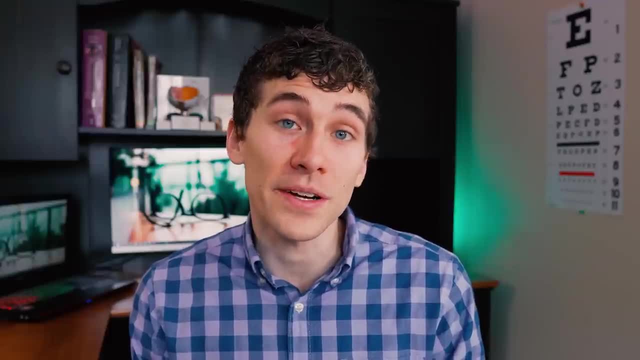 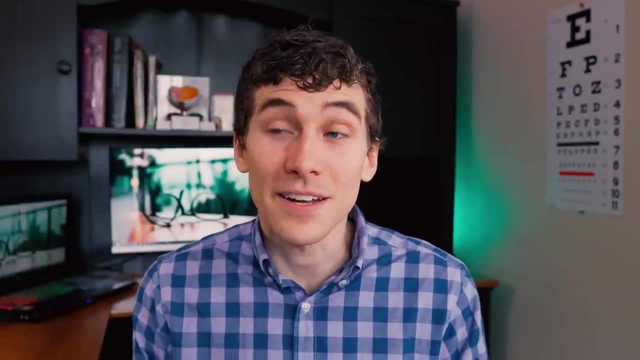 really healthy for you, the eye. In fact, some of the contact lenses on the market- especially the kind of colored contact lenses that you can find through some kind of scary online retailers- that are super cheap. They're like. I've found them online for like $5 before. Those are often made. 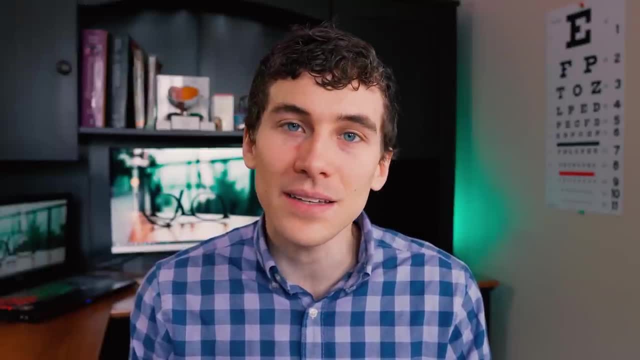 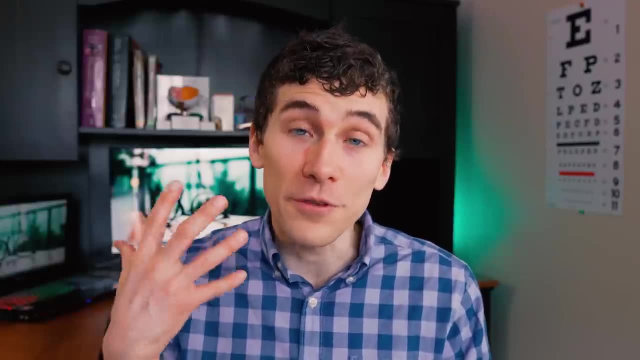 based on old technology patents from the 1960s And they're generally not very healthy for the eye because the standards for health and health for the cornea and the surface of the eye with contact lens wear weren't really available. So it's not really healthy for the eye. So it's not really. been established until the mid 1980s, But in general, for most people looking for a healthy, newer technology of contact lens expect that for a yearly supply they'd be paying about the same price of a new pair of glasses, of somewhere between two to $400.. Probably one of the biggest. downsides of contact lenses is that they do pose a higher risk for eye complications and infection, And that's why it does take some level of responsibility to take care of contact lenses and to wear them properly. That includes cleaning and disinfecting them correctly as well. 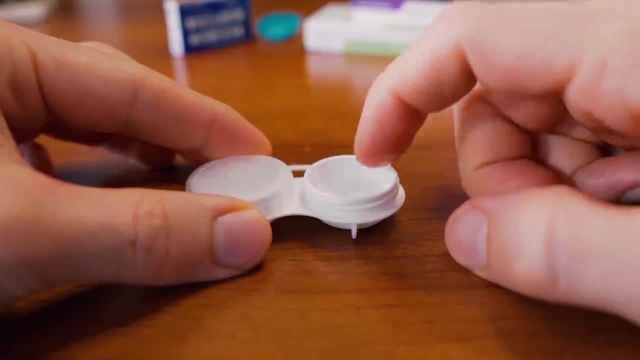 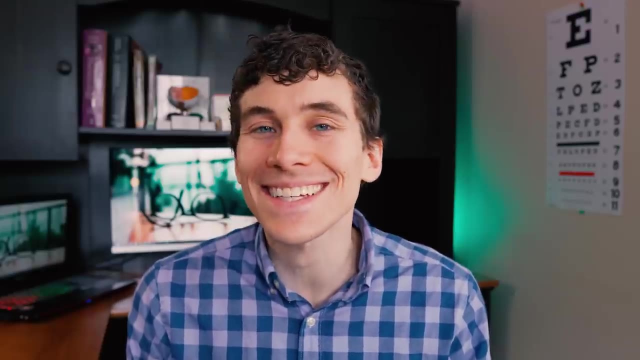 as replacing them when they're designed to be replaced. Contact lenses can also feel dry and uncomfortable for some people, especially if you already have some form of dry eye disease, And some people have difficulty getting contact lenses in and out of the eye. And if you're kind, 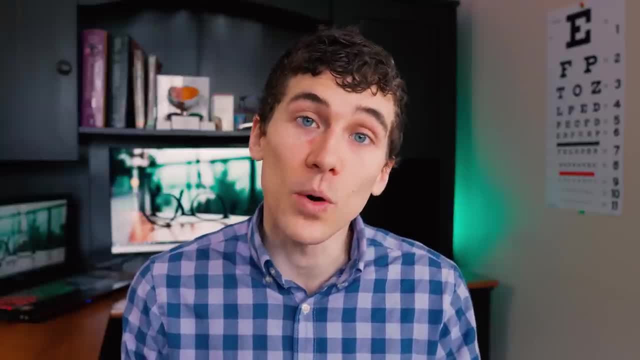 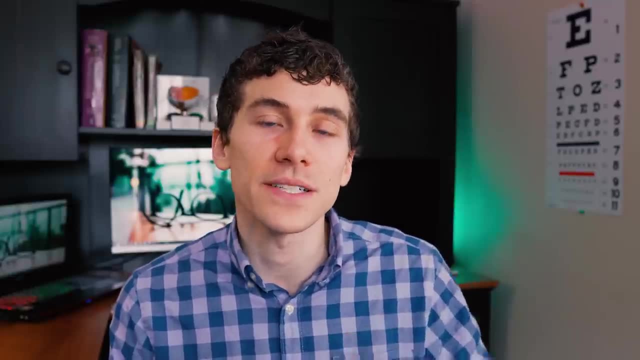 of just beginning in your contact lens journey and you'd like to kind of learn more about getting contact lenses in or out. I do have a full series kind of contact lenses for beginners. then you definitely want to check out that series And I'll hook that up in the description below. So if you're 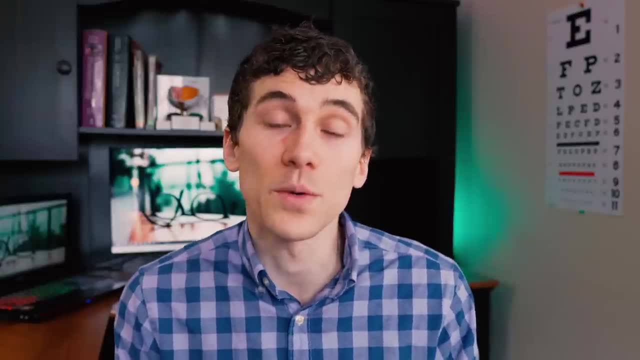 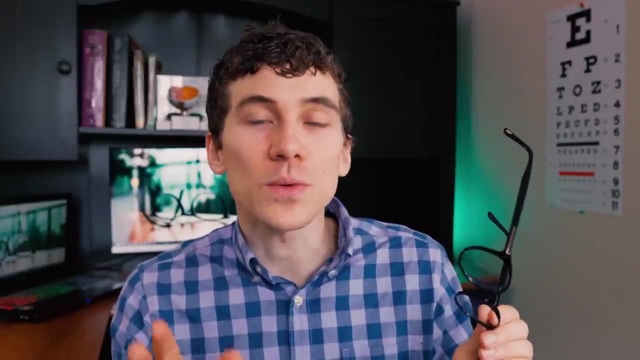 interested in getting contact lenses in, I'll leave a link in the description below for you as a resource. Now, as far as glasses versus contacts, in terms of which gives you better vision, that's a tough debate And it really depends on a couple of factors. For most people, glasses are probably. 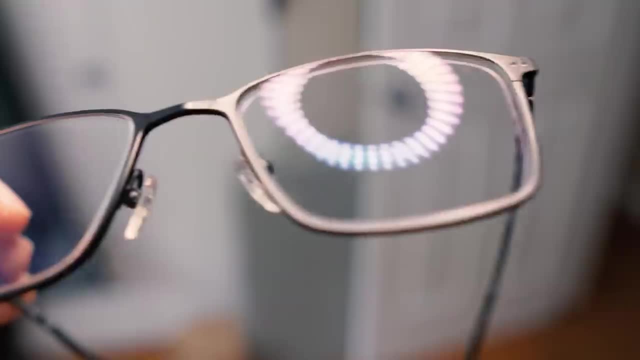 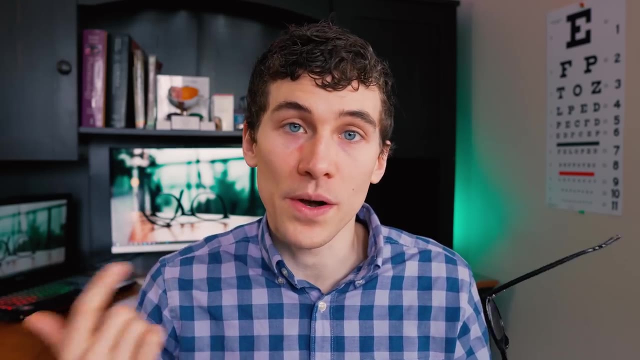 going to have a higher optical quality and will give you sharper vision. as long as your glasses are clean, they're up to date and fitting right As far as soft contact lenses go, like the ones I'm wearing now. In general, again, the optical quality is not quite hitting glasses, But if you're. 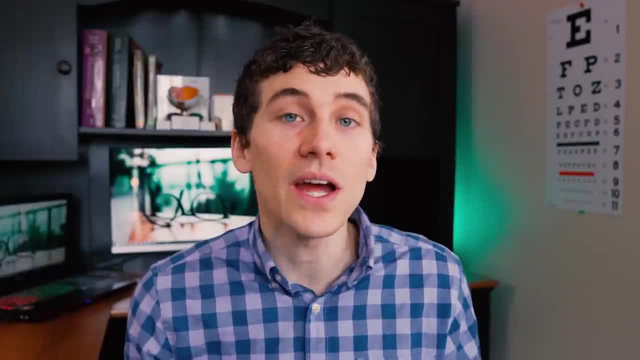 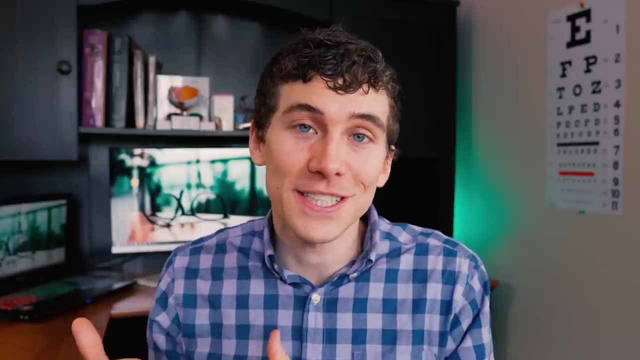 interested in getting contact lenses in and out of the eye, you're going to want to check that out. But if you're interested in getting contact lenses in and out of the eye, you're going to want to check that out. However, there are some people who do better with contact lenses versus glasses And 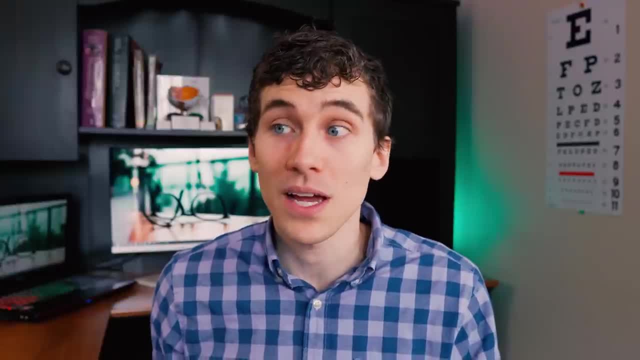 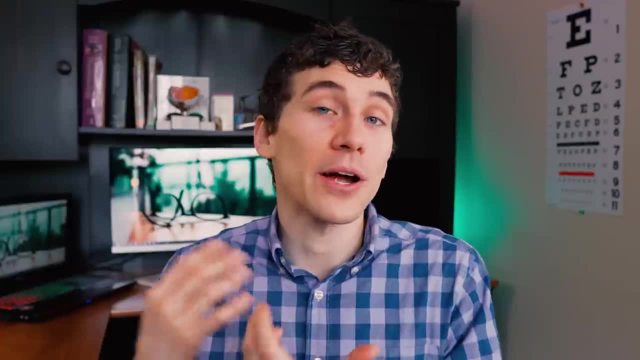 those are usually individuals who have a really high glasses prescription because with the higher prescription they're going to have more distortions in the lenses where somebody who has a kind of high amounts of astigmatism or some type of corneal disease such as keratoconus they may do. 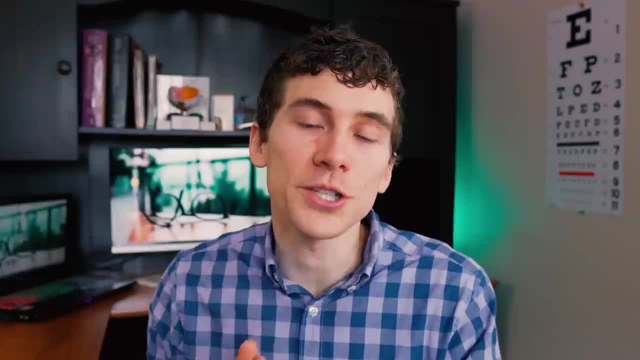 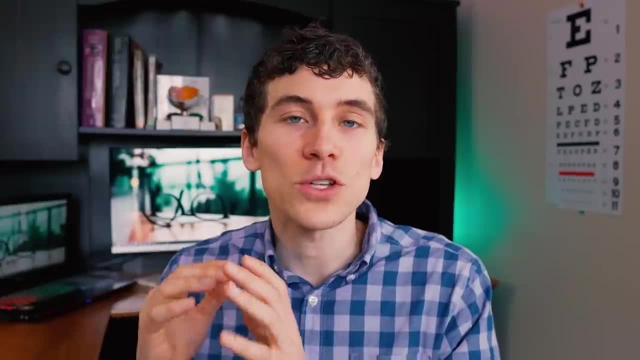 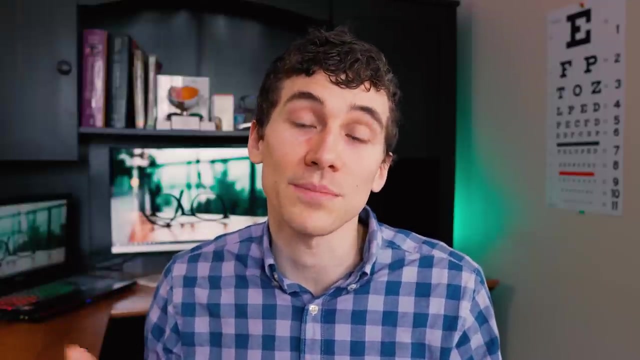 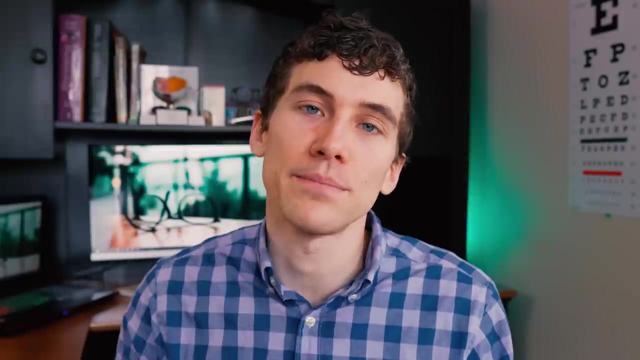 better with specialty contact lenses such as hard optical contact lenses. So if you're interested in Either that or some type of scleral lens- but in general people see a little bit better with focused contact lenses. But to answer that question, I'm going to pass it off to you. Do you prefer? 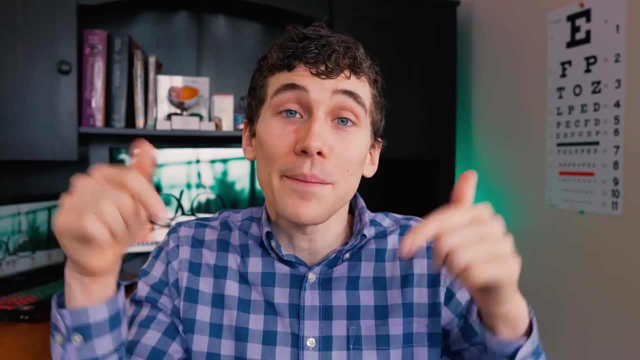 glasses or contact lenses? Which kind of contact lens do you prefer? Because that's what I was looking for. you see better out of. Go ahead and leave a comment in the section below. Hey, if you liked this video, go ahead and smash that like button for me, And if you're a glasses wearer and you 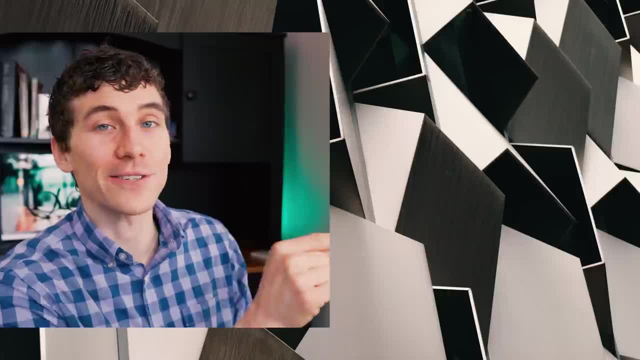 haven't seen my tips or tricks for glasses wearers, go ahead and check out that video by clicking or tapping the screen up over here to the side. Or maybe you're getting into contact lenses and you'd like to learn more about those. For that, you can check out this video series. 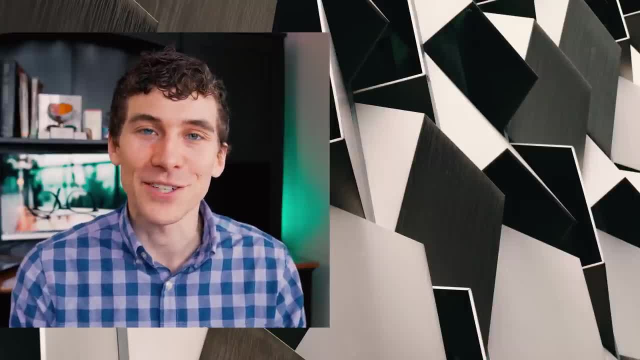 down over here. Again. this is Dr Alan here, helping you with the eyes and vision. Keep an eye on it. We'll talk to you soon.